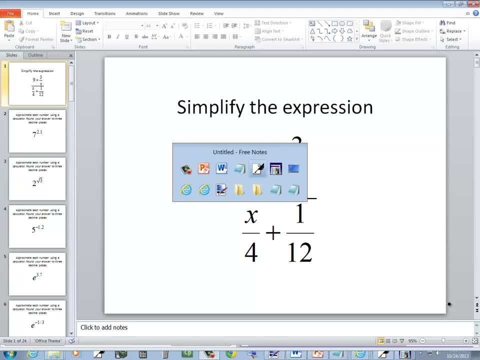 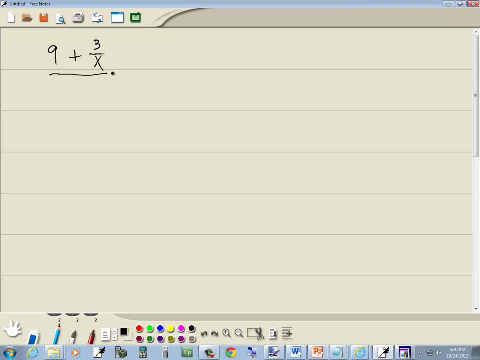 Let's simplify this expression. We've got 9 plus 3 over x, all over x over 4 plus 112.. Now, this is a complex fraction. This x, right here, this is an inner denominator. This 12 is an inner denominator. 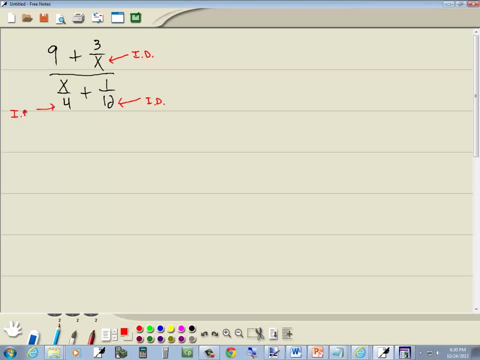 And this 4 is an inner denominator. These are fractions inside of a fraction. That's what complex fraction means. Now, specifically, when you have x's, they refer to it as complex rational expressions. But again, we have a fraction inside of a fraction And it's got its own denominator And I'll refer to that as the inner denominator. Now what we're going to do is we're going to multiply everything by the LCM of all our inner denominators. 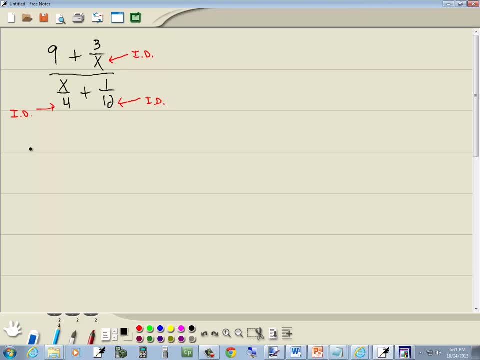 Well, let's first look at the numbers 4 and 12, the LCM of that. So this would be 12.. And the x, since I just have a single x, then my LCM total would be 12x, And that's where we're going to multiply it times everything. So I'll multiply it times a 9.. I'll multiply it times the 3 over x, I'll multiply it times the x over 4.. And I'll multiply it times the 1 over 12.. 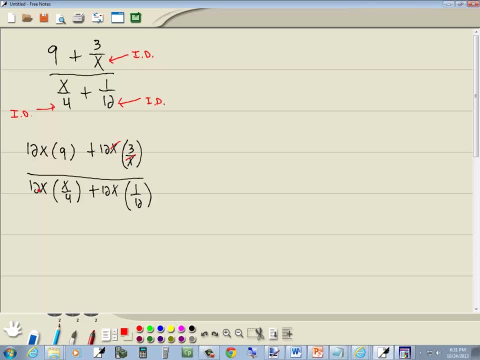 Well, these x's are going to cancel here Now. here we've got 4 and 12, both of those by 4.. 4 divided by 4 is 1.. 12 divided by 4 is 3.. Here we've got 12 and 12, both of those by 12.. 12 divided by 12 is 1.. 12 divided by 12 is 1.. 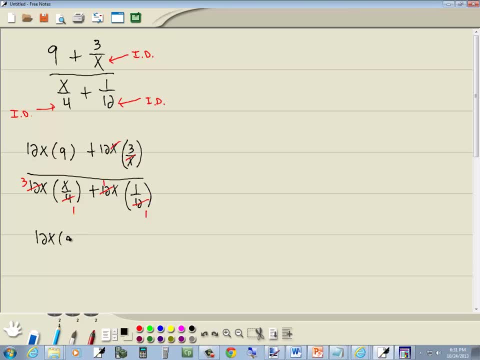 So we're left with 12x times 9 plus 12 times 3 over 3x times x. So the 3, the x and this x Plus these 1's don't do anything, so I'll just write an x. 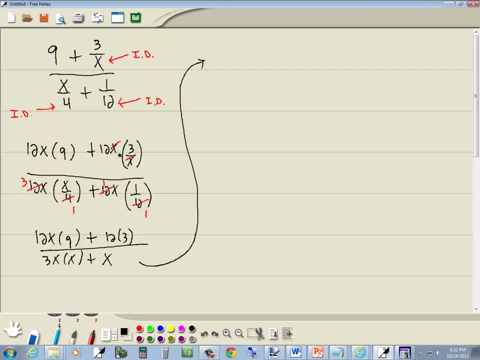